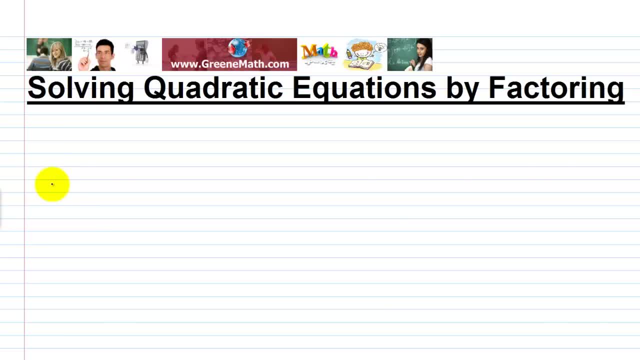 to get a solution in some cases. So you're going to get some easy cases where it's going to be possible to factor your quadratic and then you can go through and get a solution. So that's what this video is going to be about. So, basically, let's start out by giving an official definition. 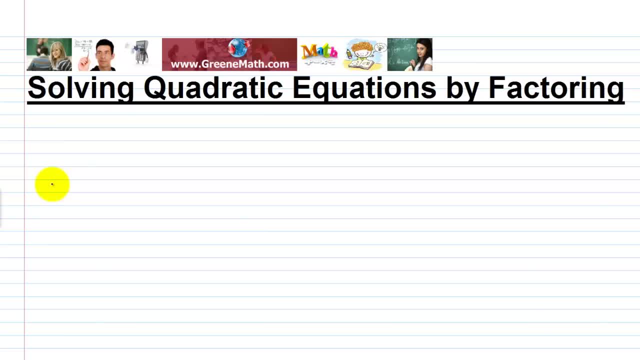 for what a quadratic equation is. Now we've been working with these when we've been factoring. But basically a quadratic equation is a quadratic equation Contains a squared term and no term of higher degree. Okay, so kind of: contains a squared term. 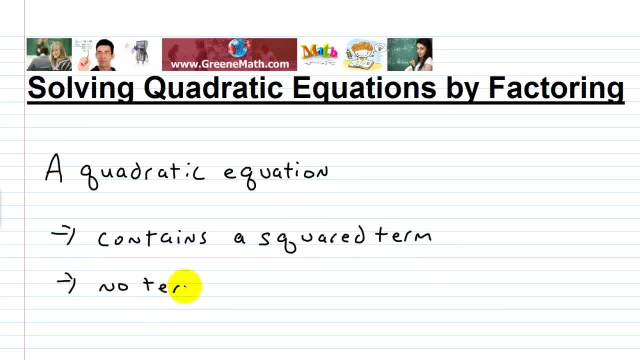 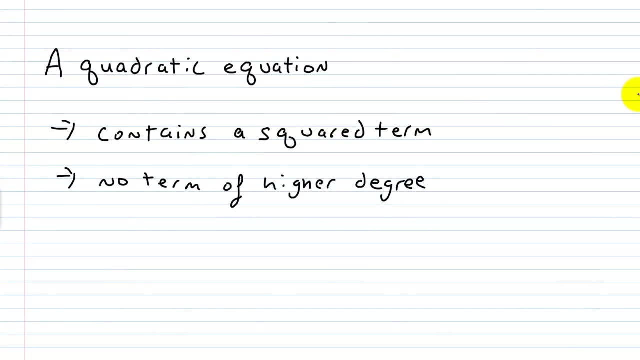 And it has no term, No term of higher degree. So basically, when we were factoring, we kind of wrote out this generic quadratic equation which looks like this: Ax squared plus bx plus c, right Where we said that a was any. 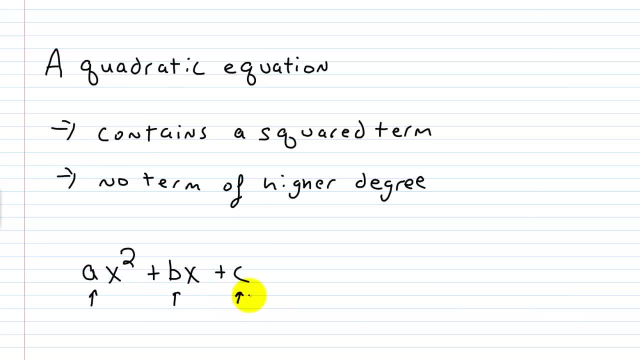 real number, b was any real number and c was any real number. Well, here we have a condition: that for us to have a quadratic, a cannot be a quadratic be equal to 0. And the reason for that is because we have to have remember this criteria that we 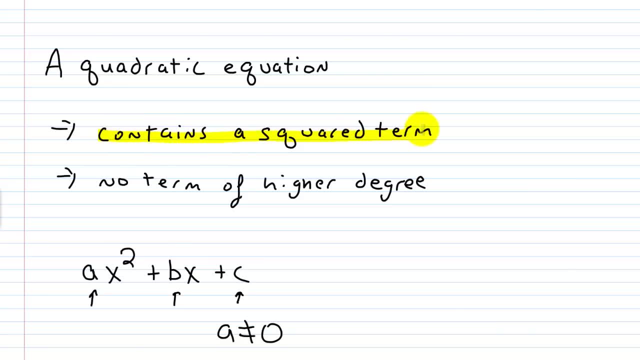 gave, it has to contain a squared term. okay, So if a was to equal 0, you'd have 0 times x squared and that would be 0. So a cannot be 0 if you have a quadratic equation, So something that's called. 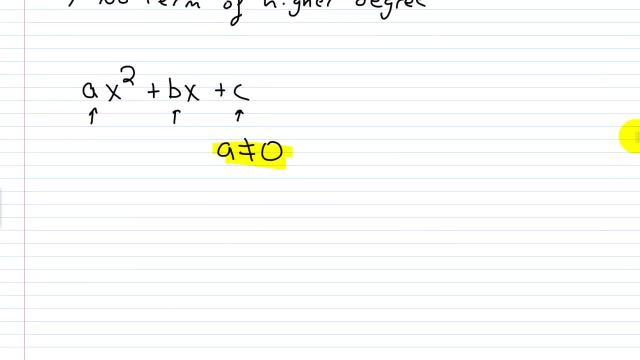 the standard form. okay, the standard form looks like this: It's ax squared, okay, ax squared plus bx plus c, and then now we have equals, because we're dealing with equations now. so equals 0.. So this is the standard form for a quadratic equation. You want it to kind of look like this: 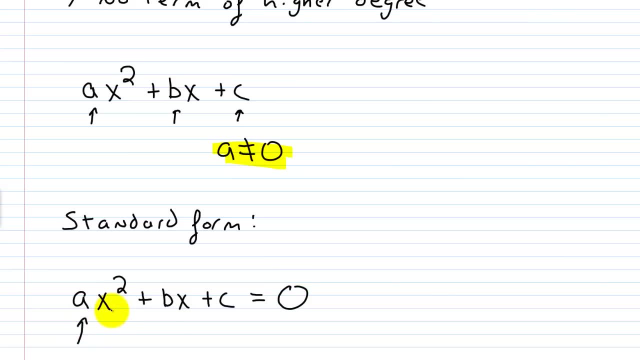 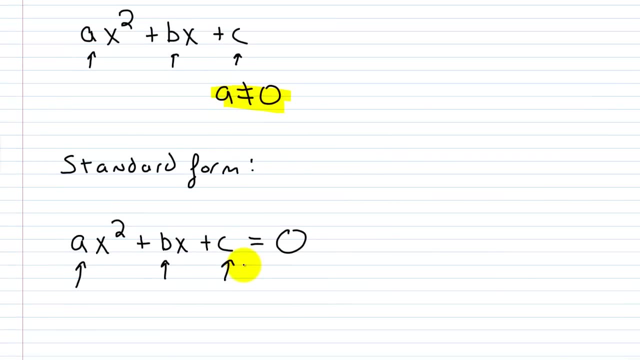 equation. Exactly So you'll have some coefficient for your x squared a coefficient for x and a constant term hanging out by itself. And remember, the restriction is that a cannot be equal to 0.. b and c can be 0, okay, but a cannot be equal to 0.. 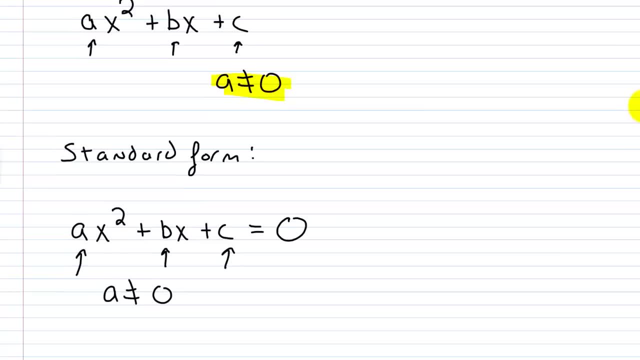 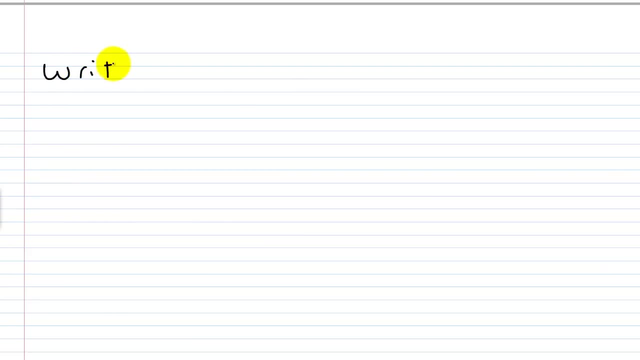 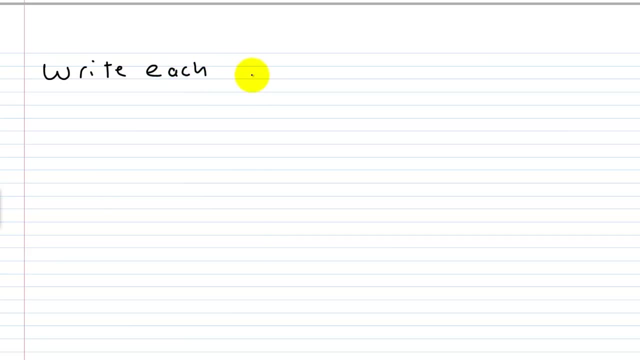 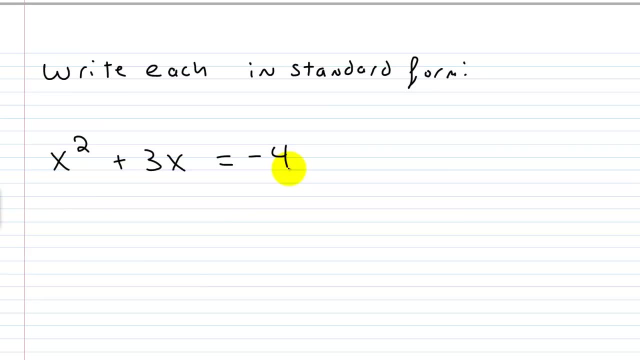 So how do I put that in standard form? Well, basically we're just going to use some properties that we learned about when we're studying equations to kind of move this into the format of what Ax squared plus bx plus c equals 0.. 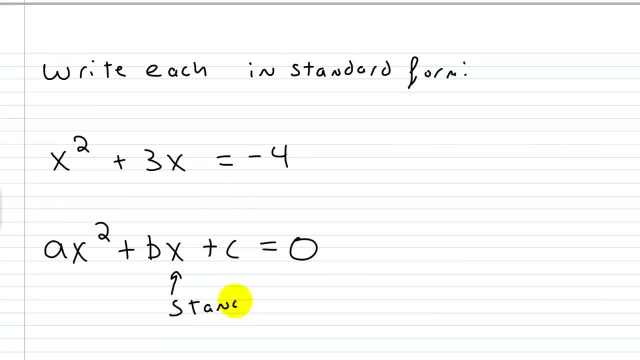 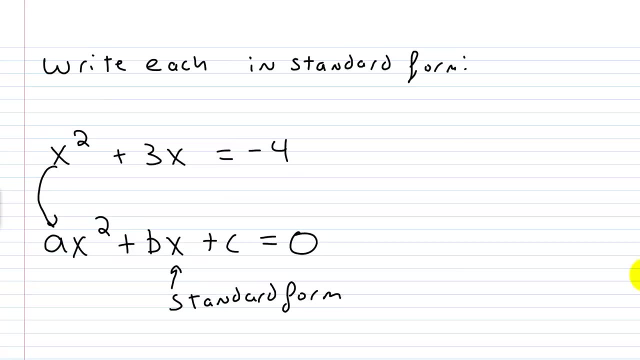 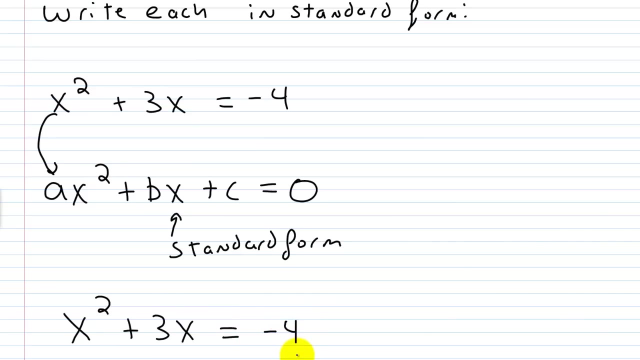 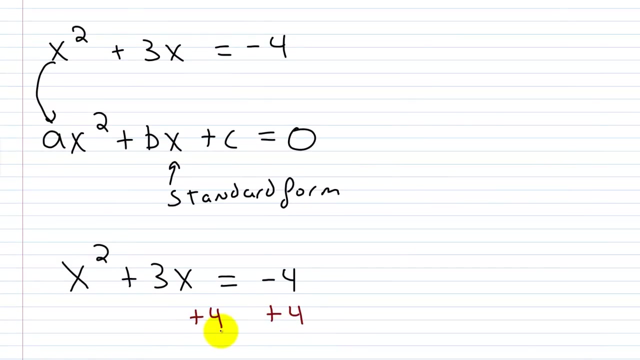 That's my standard form. So how do I get this to match this? Well, let me just rewrite this: x squared plus 3x equals negative 4.. Well, I know that if I add 4 to both sides of the equation, what I'm going to end up with is negative 4 plus. 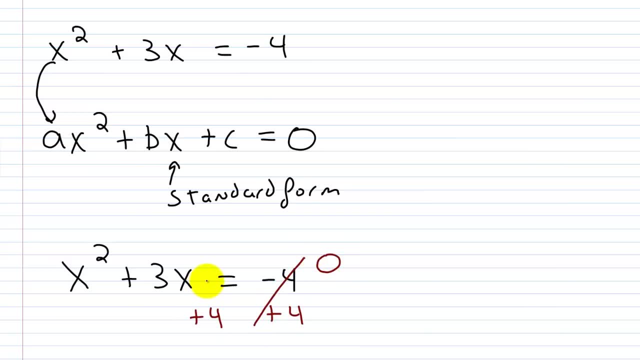 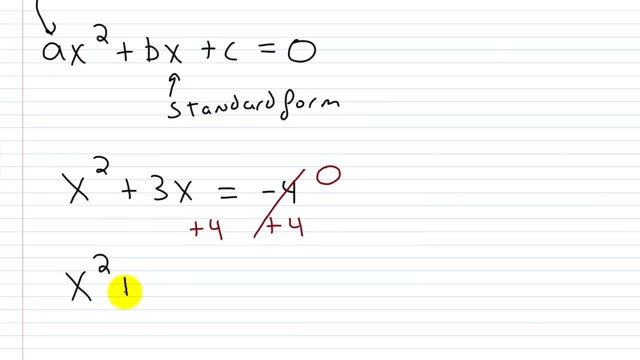 4 is 0. So this would be going to be 0. And then I could just put a 4 at the end of this left side here, and I'd end up with x squared plus 3x plus 4 equals 0.. 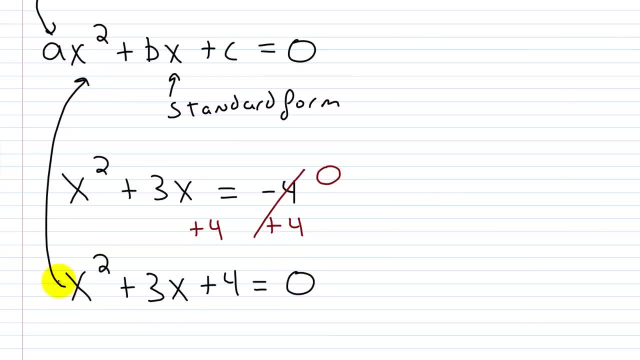 So this is exactly what I have right here: a equals 1 here. so I have basically 1x squared plus 3x. This is basically. I'll put- This is my a term, it's kind of a 1.. 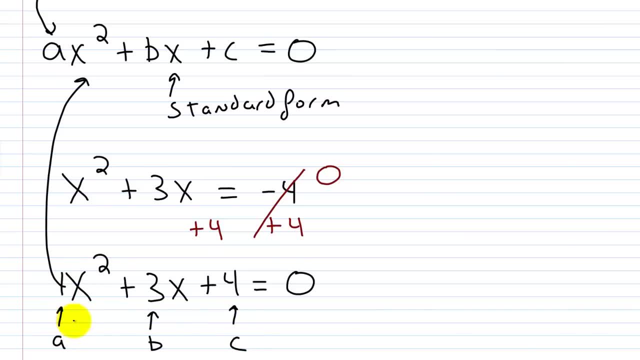 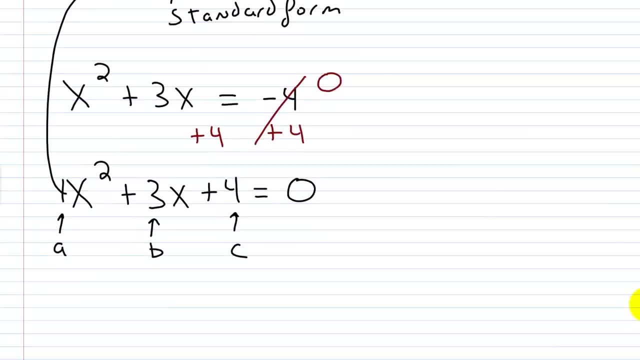 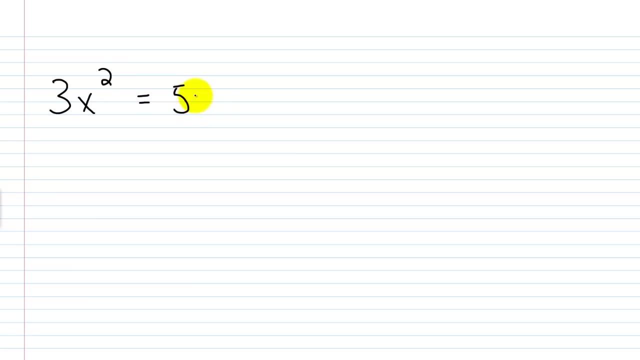 This is my b term, and then this is my c term. So I have ax squared plus bx plus c equals 0, and that's exactly what I want. Let's look at another one. Let's say I gave you something like 3x squared equals 5x plus 7, and I want to write this: 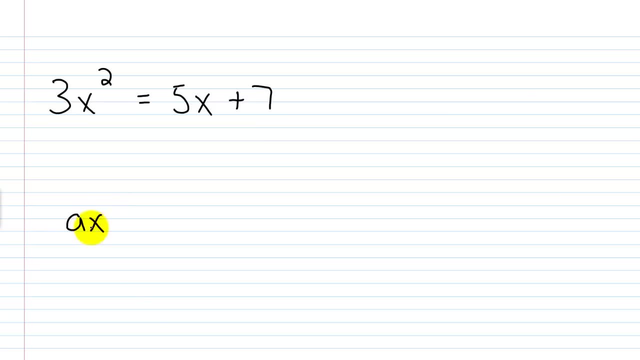 in standard form- and remember, standard form looks like this: ax squared, squared plus bx plus c equals 0, okay, So what I'm looking at here is I have this over on the right side and what I want to do is just move that over to the left side and I'll have something that matches this.